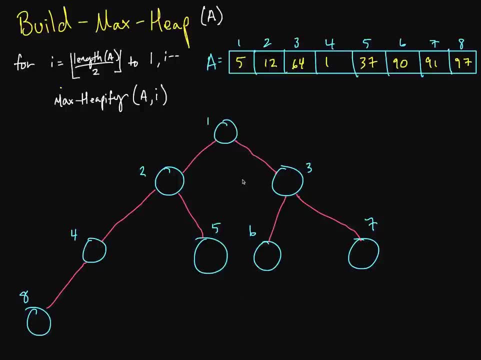 Welcome to our 15th video with data structures and algorithms, And in the last video we talked about how to do a max heapify, And in this video we're going to talk about how to actually do build heap and how we're going to actually implement a heap, Because last time we did. 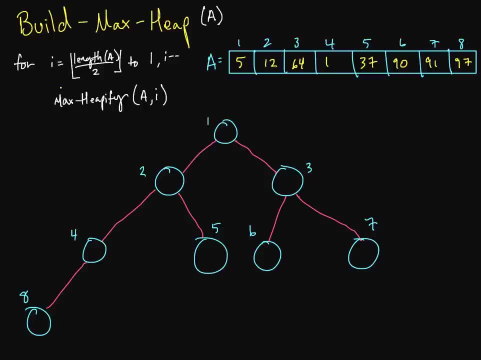 we just had this arbitrary tree- you know this binary tree- with a bunch of nodes in it, And then we called max heapify on that and built a max heap out of that or turned that into a max heap. Now we're going to use an array right to store a heap And it's 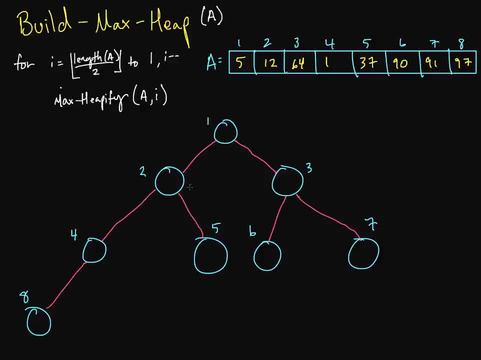 easier for us to do that right. We don't need to actually do like a linked kind of a list right where we have like pointers, because this actually that when we draw these trees it kind of looks like we have you know. 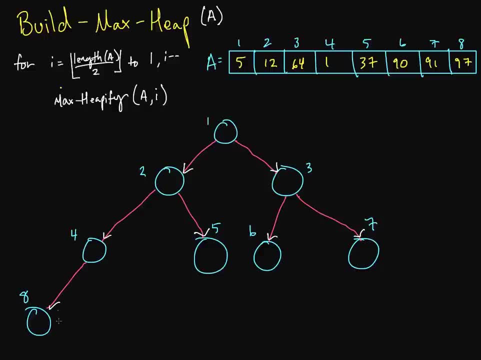 Pointers right to these other elements. Visually, we kind of it's easier to think of it that way, But we can use an array which is a little bit more efficient, right, We don't have to worry about that stuff. So how do we build a heap out of this array? Well, 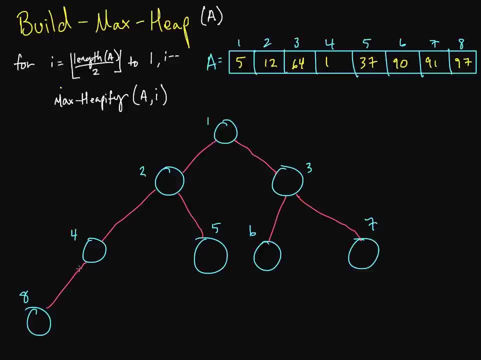 I've marked all these nodes. okay, We've got eight elements in our array. so we've got eight nodes And I've marked each one. Now we have to keep the nearly complete property of a build heap. So if we just number these from top to bottom, left to right, okay, 1, 2, 3, 4,, 5,, 6,, 7,, 8,. 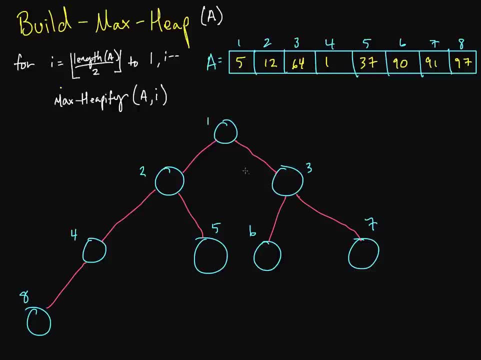 we keep that property right. So there's our first thing, And all we have to do is insert these elements, right? We're not really inserting them, but in our visual diagram here we're just going to write these elements here, right? So we've got 5, and then 12, and then 64, right? 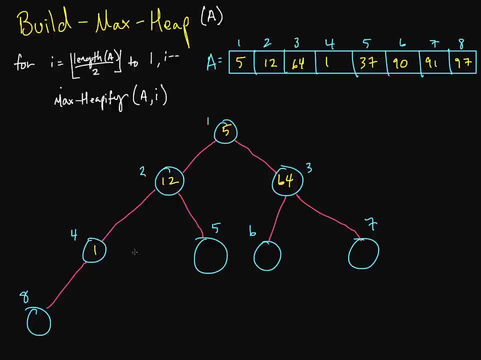 We're just going along Left to right, right 1,, 37,, 90,, 91, and 97.. And now here's our little algorithm, right? So we're ready to actually build heap. All right, so we take this right from length. 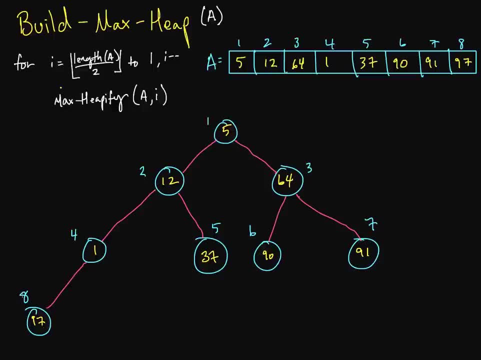 of A, the last one, the last element, and we divide that by 2.. And then we max heapify from there And, as we said in the last video, we start from the last subtree which is here right, It just happens to have one child element, And then we go to this one right, One less. 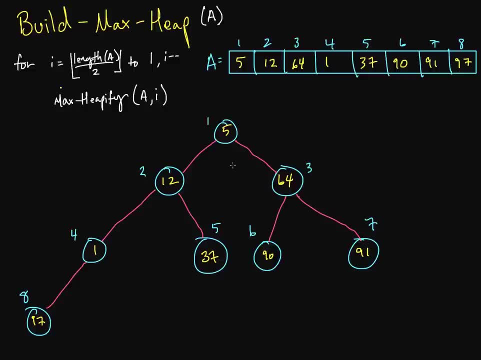 right 4, minus 1, minus 1, minus 1, right, And we heapify, we max heapify each one of these subtrees, okay, So that's what we're going to do. So I equals 8 divided by 2, minus. 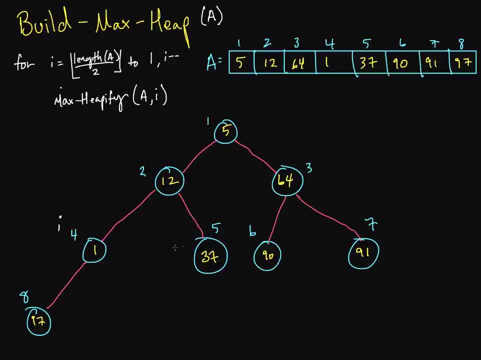 floor. So I is here, okay, And we max heapify And, as we said before, we take the larger of the two child elements and we swap with the parent, okay, That's if the parent is, of course, less than or equal to the children. So in this case we've got to take 97, right. 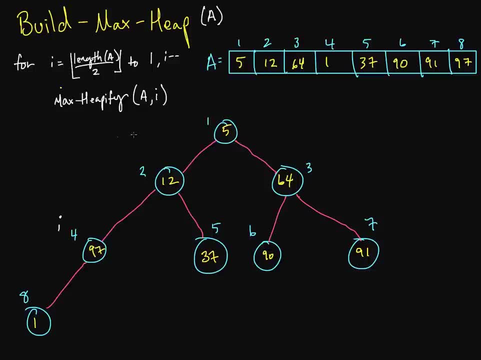 97 and 1 and swap those two And now we're done with our max heapify there. So I gets decremented right And now I is over here, So let's max heapify this. So both children are clearly greater than right the parent. 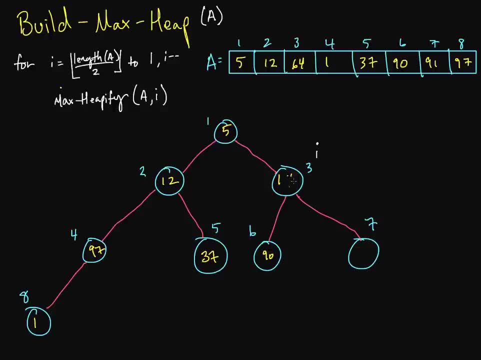 node. So we take the larger of the two, which is 91. So 91 and 64 get swapped And we decrement i okay, And what I should be doing is swapping these right. So 97, and where did I draw this? 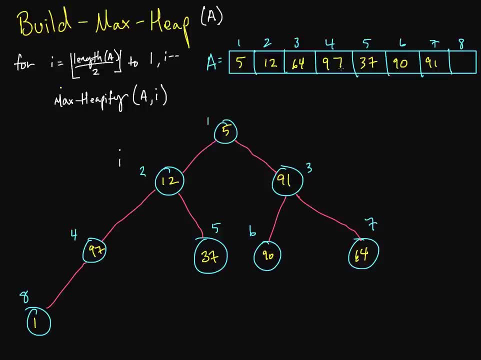 97.. 91.. 91 got swapped, And then 64 and 91 got swapped, right 64. Okay, And now we're here on this one. So what we have is both of these are greater right. So 97 is the greater of the. 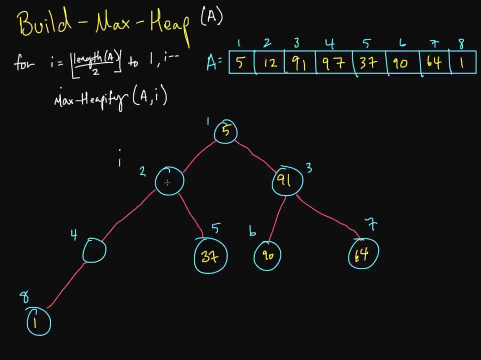 two. So we take 97 and 12.. 98.. 97 and 12. And we'll do the same thing over here. All right, this was 97. And this should be 12.. Okay, so now that one's done And we'll decrement i. Okay, And we need to swap right. 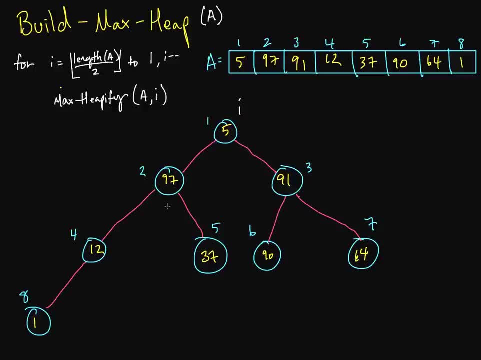 Because clearly both children are less than- And we didn't screw up the max heapify here, right, So we didn't have to fix that one: 98. 98. 98. 98. 98. So here 97 is the greater of the two, so we'll swap that. So this is five and this. 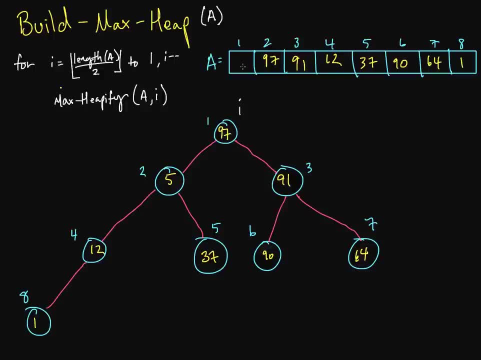 is 97.. Let's just reflect that up here. So 97 and five right, And now we have kind of destroyed the property here or not there, but right here- of the parent being greater than or equal to 99.. 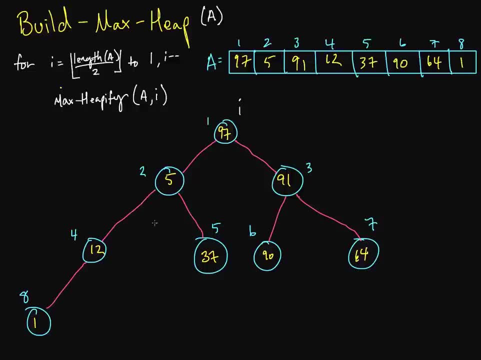 to its child nodes. so we gotta max heapify this one. So here the larger of the two is 37. Right, so we swap those two and we will reflect that over here. So 37 and five. 37 and five swapped. 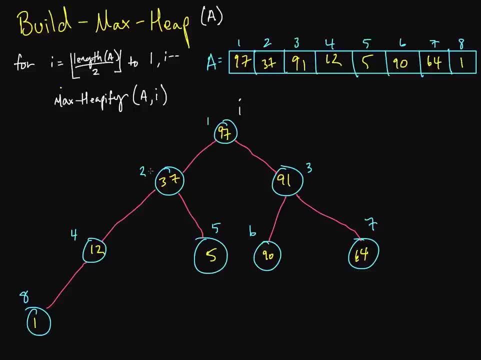 And now we should have a max heap. So let's check: Is 37 and 91 less than 97? Yes, Is 12 and five less than 37? Yes, Is 90 and 64 less than 91? Yes. 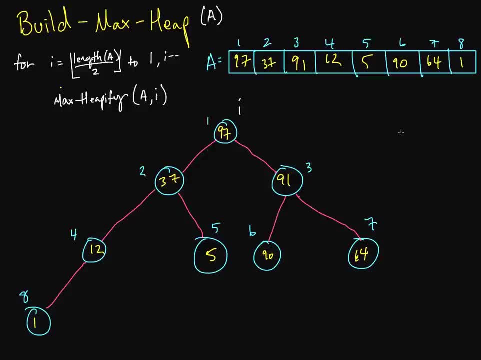 Is one less than 12?? Yes, And we have successfully built a max heap.